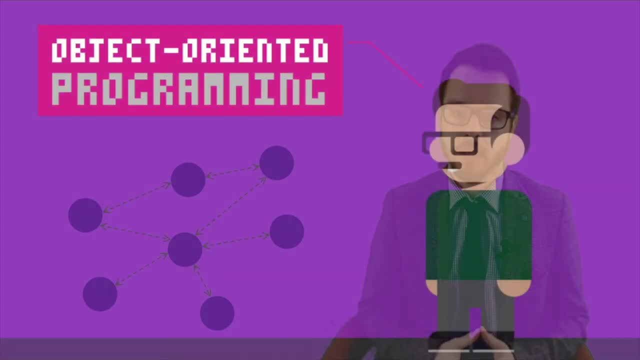 25 years is object-oriented programming right? So I think it is important for us to stop for a moment And, before we start showing some Lua code that works with object-oriented programming, I will try to, in five or 10 minutes, do a quick review of what object-oriented programming 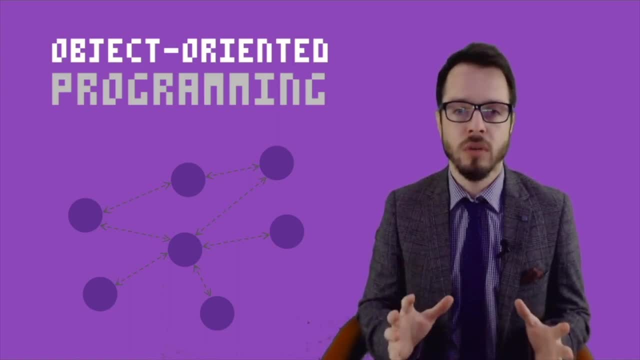 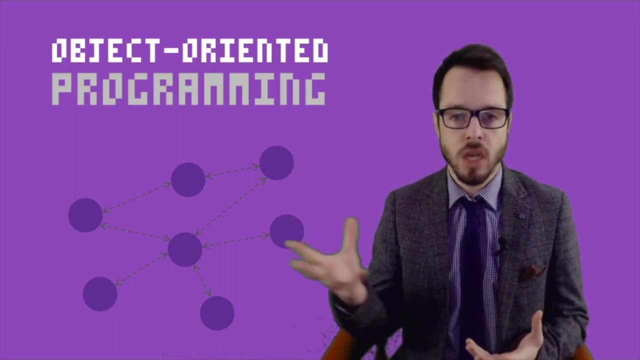 really is, Because I want everyone to be on the same page and I'm going to start using some terms, some names, some jargon, right? So whenever I use this jargon, I want you to be aware of what they mean. in the OOP, right under the umbrella of what we call object-oriented programming, 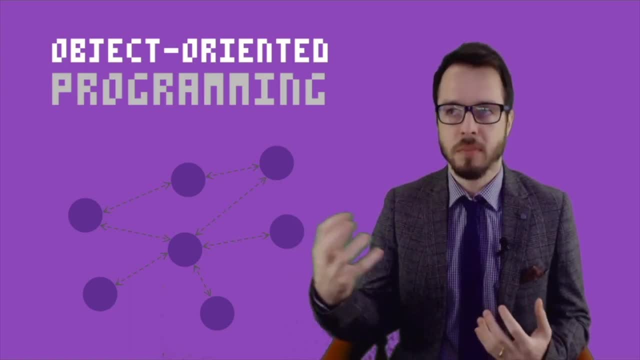 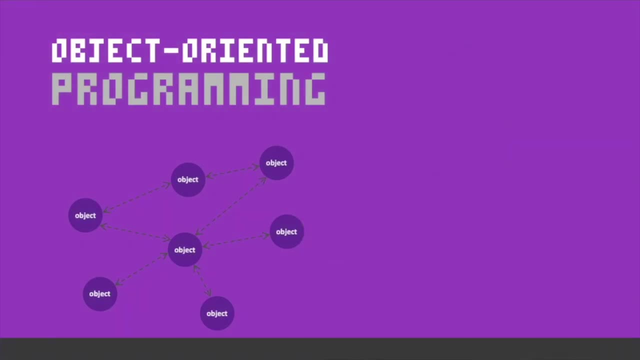 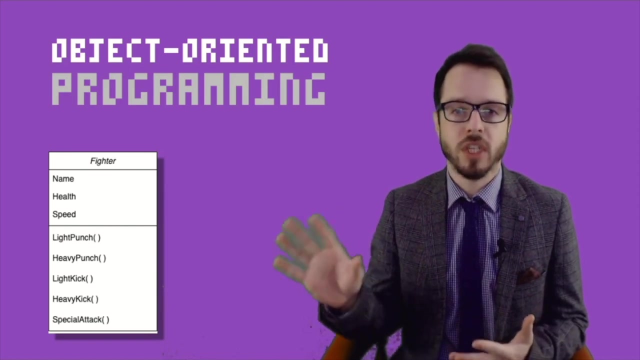 Okay. so instead of using this function, parameters and variables, we're going to have this kind of self-contained objects, And these objects are going to communicate with each other. So before I start, I'd like to just give an example of what I want to use, so we can maybe understand what objects are giving and putting things into. 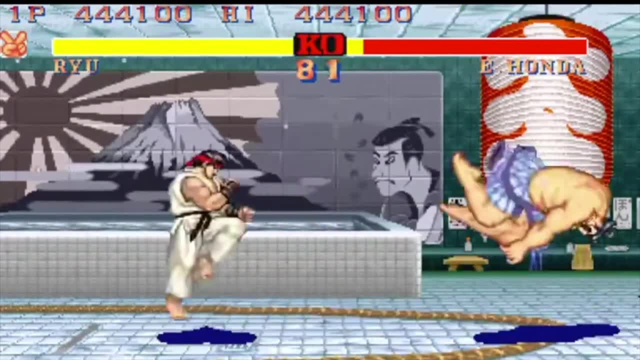 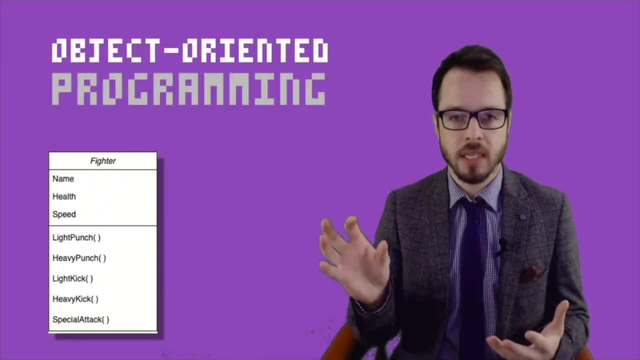 context right. So do you remember I spoke to you and I kind of mentioned a game called Street Fighter. So Street Fighter is a very classic game that you can select the player, you can select a fighter that you want to fight with, and then you go, they fight with each other and then you can kind of punch, you can kick. 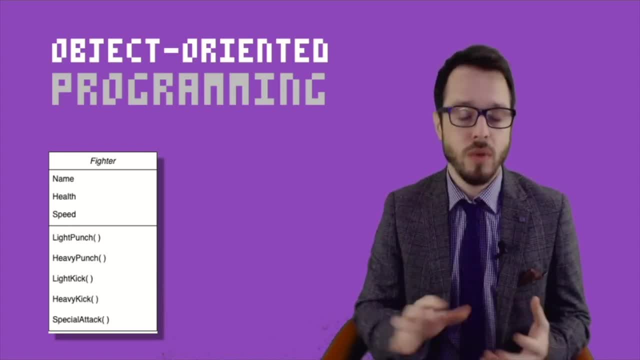 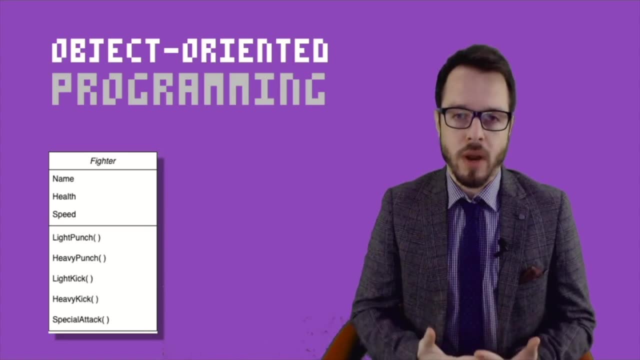 you can do all this little. give a special attack, move right. So we have all this idea of a traditional fighting game Whenever we start thinking about object-oriented programming. object-oriented programming started as this attempt of making software engineering, making software development. 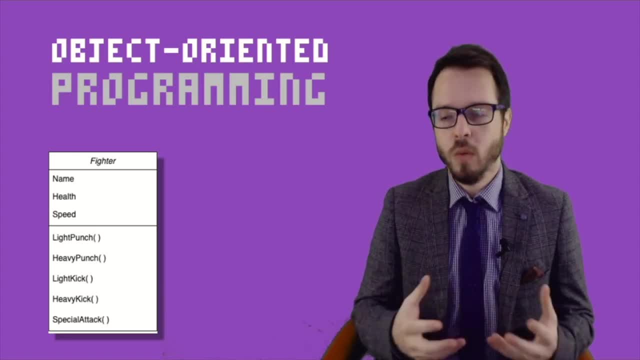 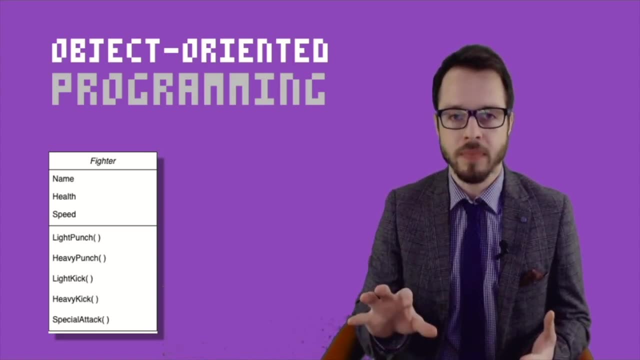 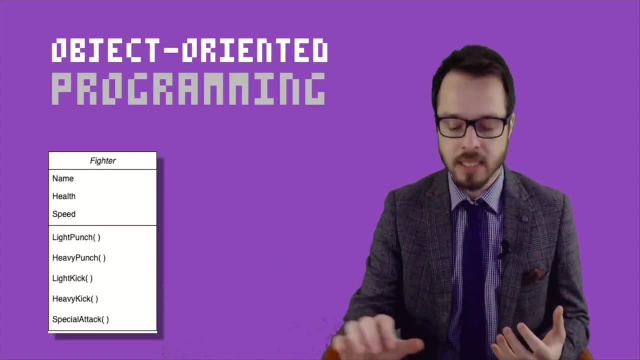 more human-friendly, right? So we with object-oriented programming, we are going to try to talk about software components and all these ideas of software elements as real-world objects, right? So you see these instances that you have in the real world, things like a desk, a laptop. 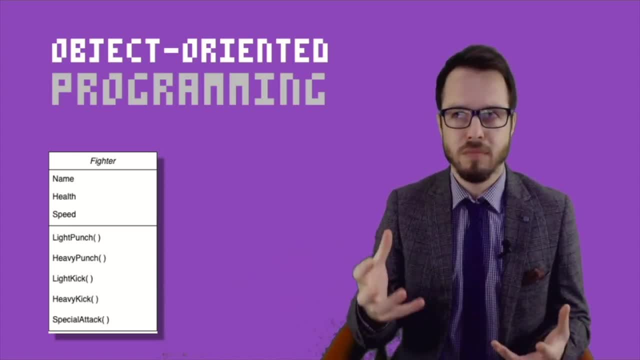 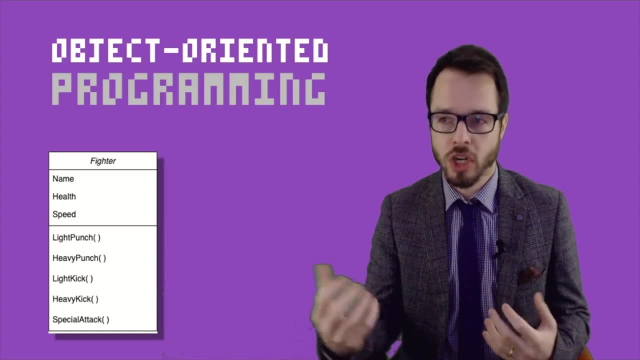 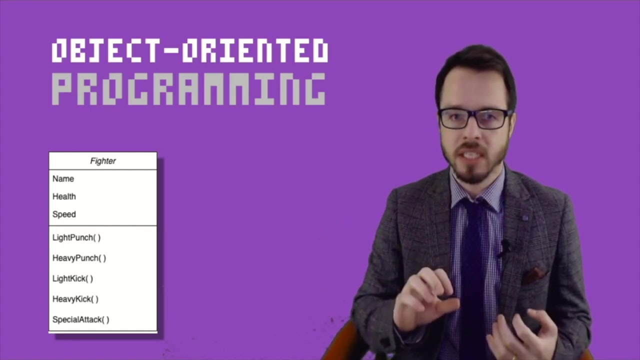 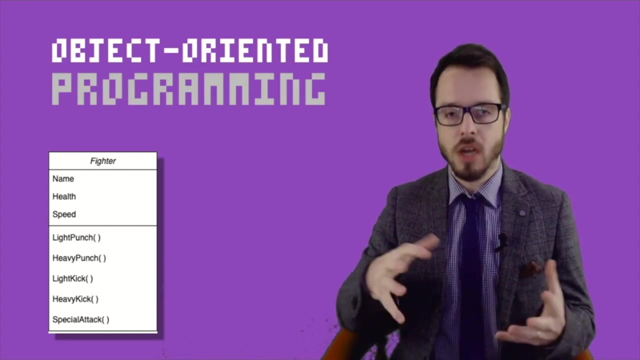 a mobile phone, a monitor or even kind of more abstract ideas of student, teacher, bank account, customer order, items, product. We are going to start to think about these elements not as a variables, not as string, integer, numbers, text. We think about them as self-contained objects. 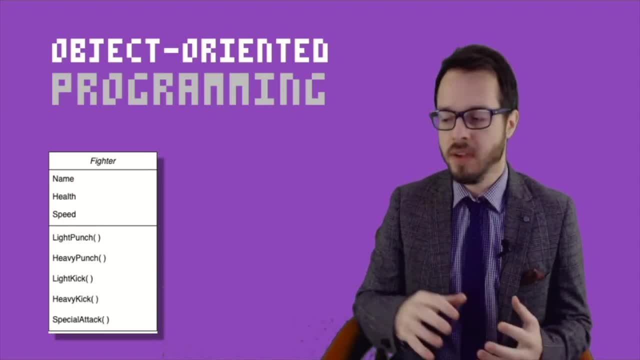 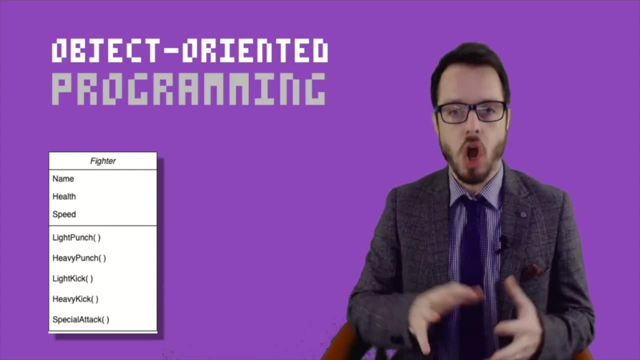 right? So I have a student object, I have a desk object, I have a bank account object, And whenever we talk about these ideas of objects, we have to remember, right? So if you go back to our example of our street fighter, do you agree that we have? 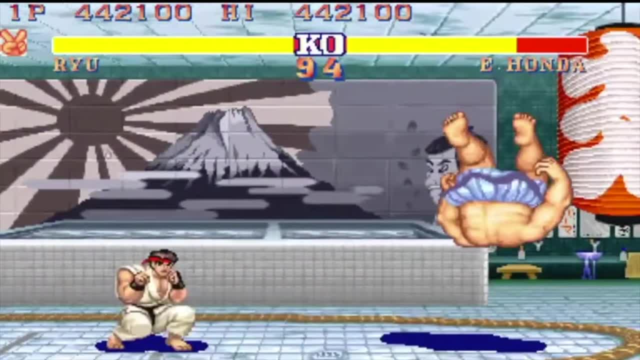 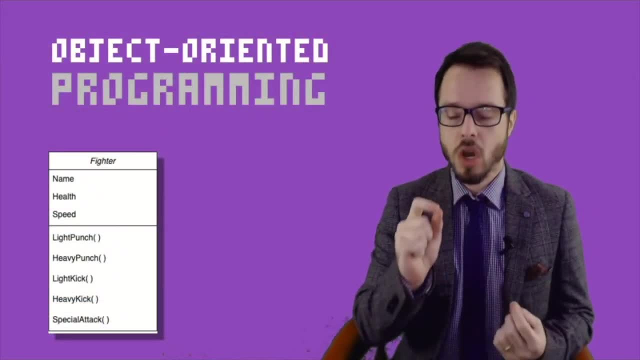 the little fighters in the game. Each fighter can be thought of as an object, right. So. So whenever I say an object, you have to remember this thing. This is super important. Objects in this OOP paradigm, right In the object-oriented programming paradigm. 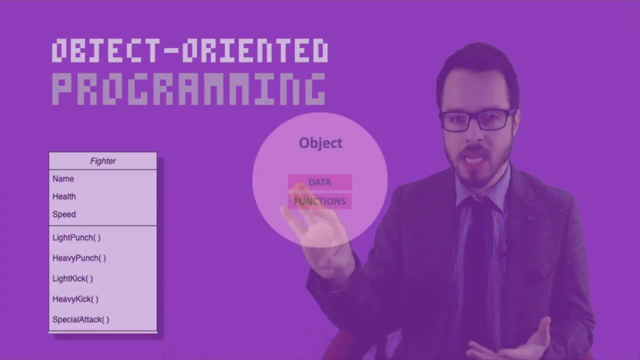 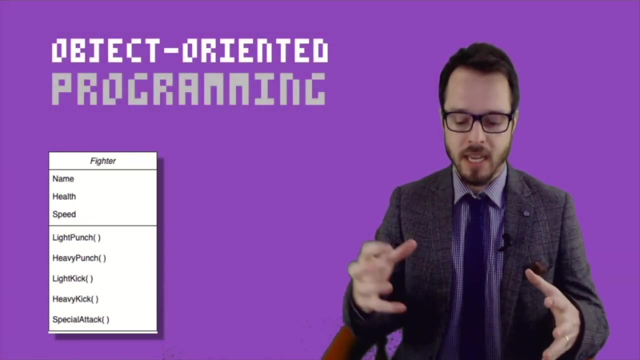 objects are basically a collection of data and functions, right? So it's almost like I put together in a little object bowl and I say here is the data of this object and here are the functions that the object can call to manipulate the data. 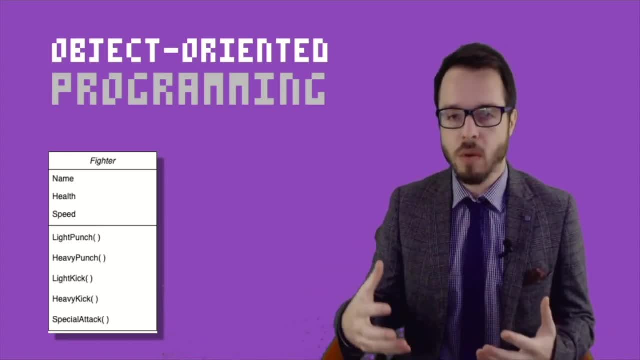 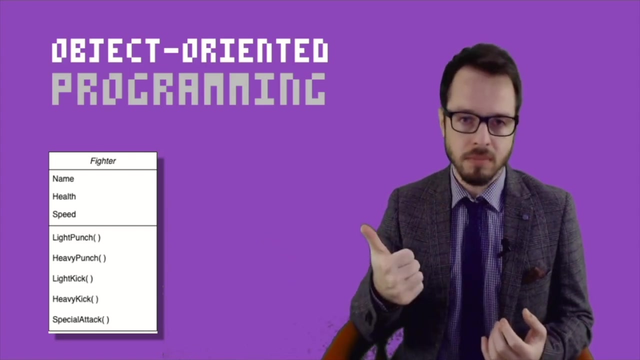 So if we stop and we look at our example of our fighter, do you agree that every little fighter that I have right in my game, every little player that I can select, this is going to be a fighter object and every little fighter object they can have a name right? 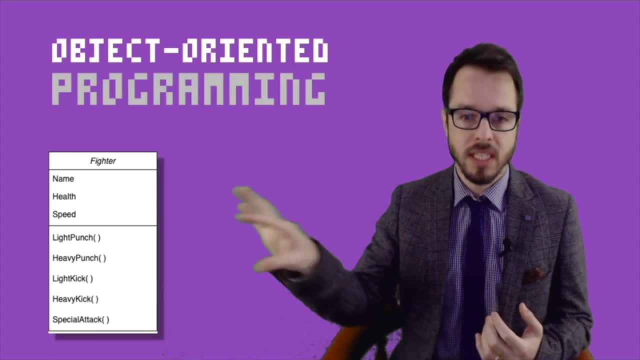 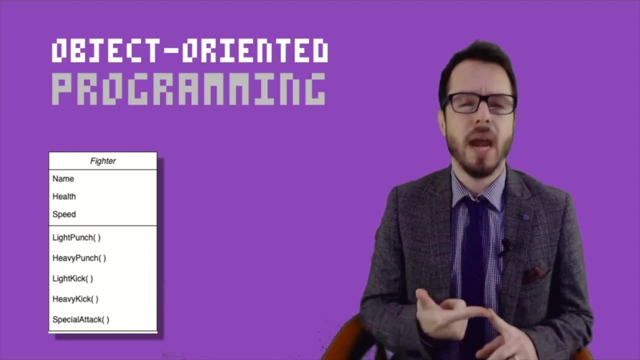 So I'm going to call them something, So they're going to have this name. This is the data, right? So this upper part is the data of my object. Name is an example of something that I can store: Health. I think about health. 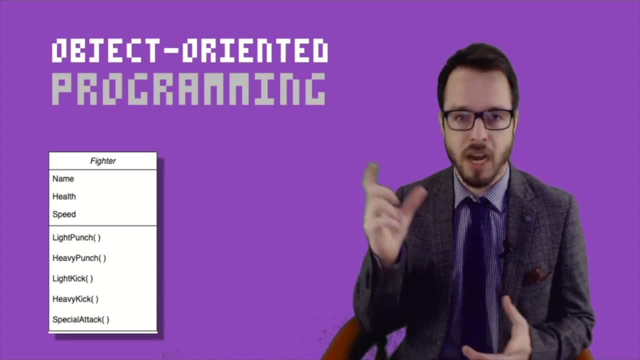 Almost like the health bar right. So what is the percentage of health that that fighter has currently? So is it 100% health, 50%, 10% or zero? So health is going to be a number data. Also the speed. 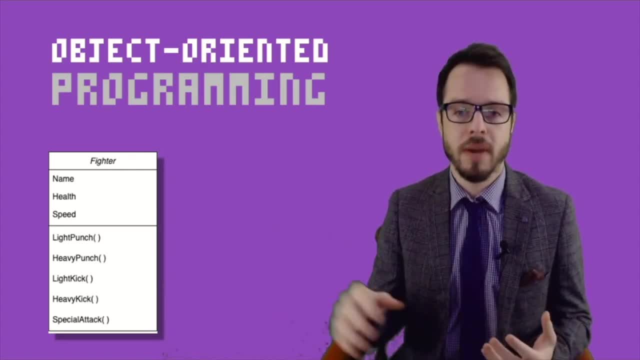 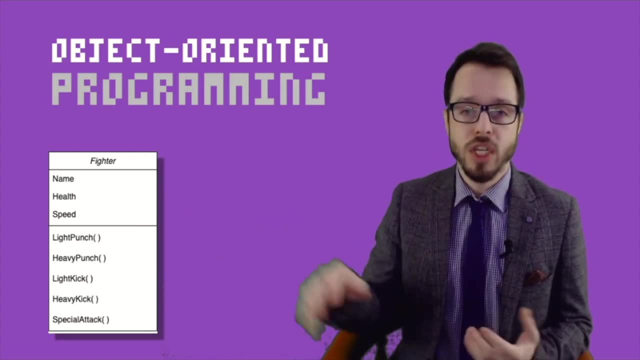 Some characters, some fighters are faster than others, right, So maybe I have a little factor of the speed there, a little number that tells me what is the speed. So this upper part right here, you will see that this is an example of 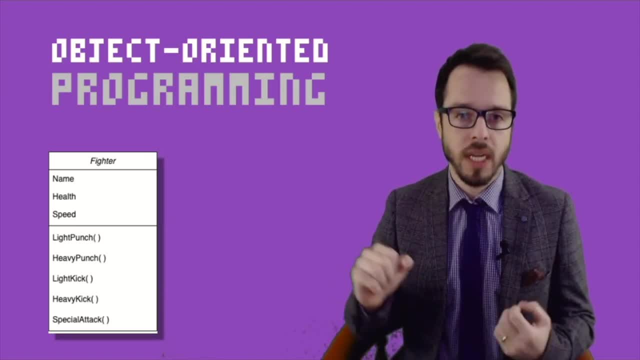 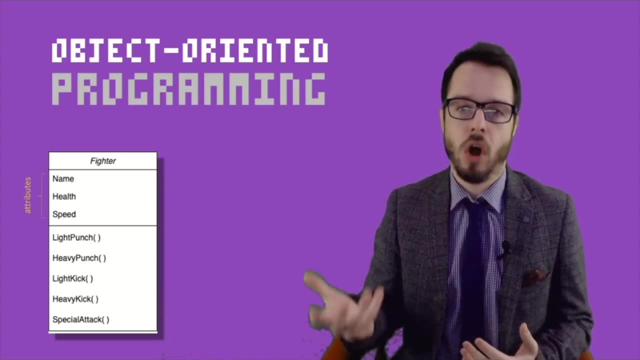 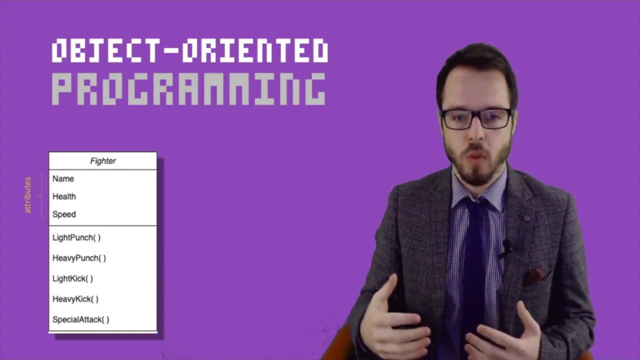 the data that that fighter object can hold inside. In the object-oriented programming world, we usually call this data the attributes of our objects, right? So these are going to be the attributes, but also our objects. in our game, We have the option of invoking and calling some functions right. 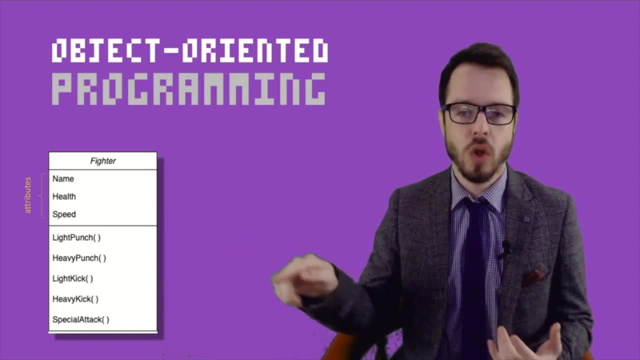 So do you agree that every fighter they could go and perform what we call a light punch? So in the Street Fighter game we had two different types of punch. So in the Street Fighter game we had two different types of punch. So in the Street Fighter game we had two different types of punch. 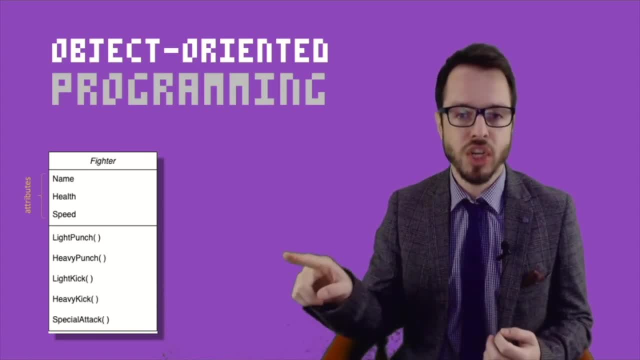 and two different types of kicks. We had a light punch and a heavy punch and we had a light kick and a heavy kick. So every fighter object in my game, they should be able to perform and invoke these functions of light punch, heavy punch, light kick, heavy kick. 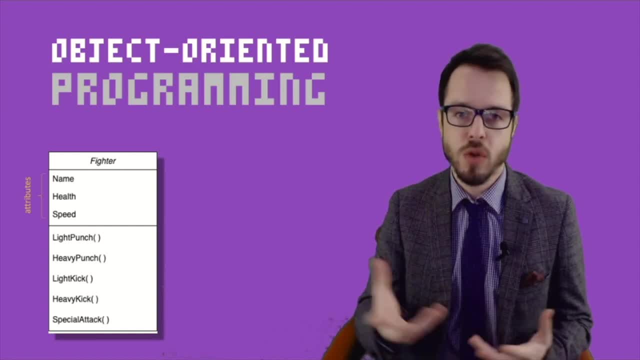 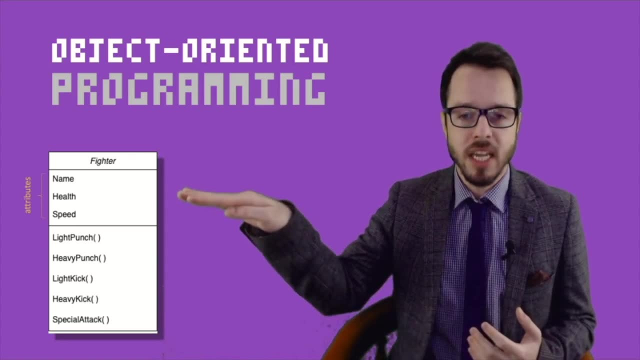 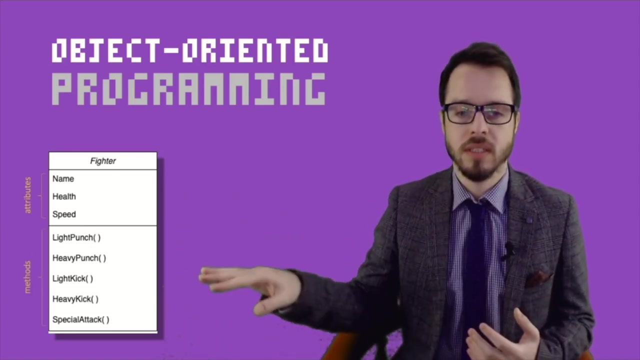 And also if they had a special attack right. So if they have a Hadouken or if they have an electric shock or whatever the special attack is for them, If this thing here was the data, if these were the attributes- here underneath I am going to list what we call these methods right. 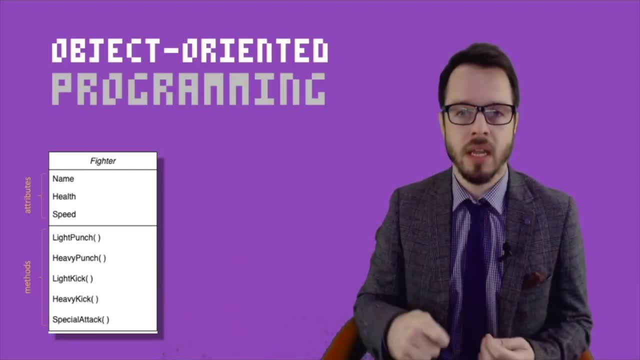 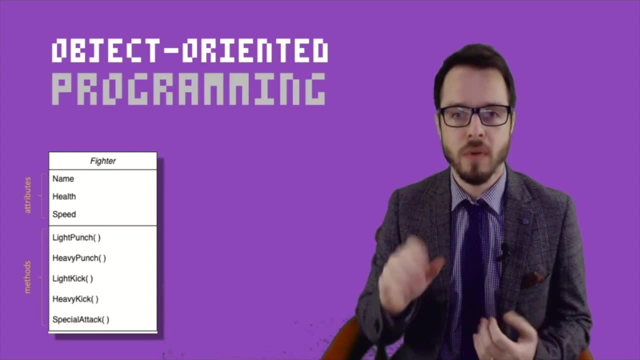 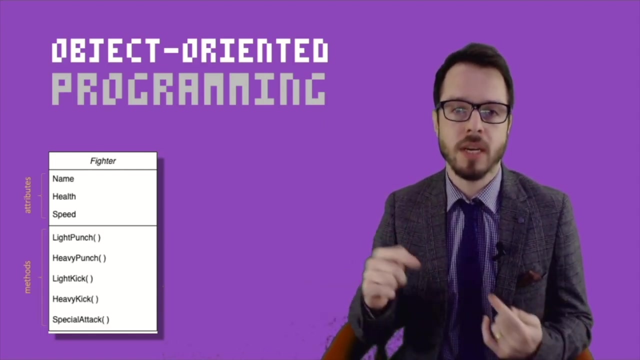 So the methods are almost like functions that our object can invoke, can call So attributes and methods right. Keep these terms always, remember always these terms, because I'm going to start ping-ponging ideas and discussing things with you by saying, oh, the object attribute, the object method right. 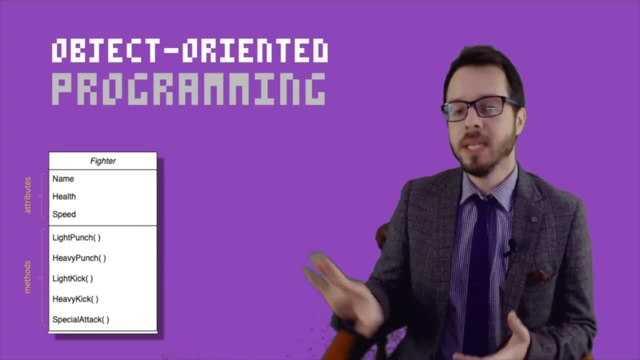 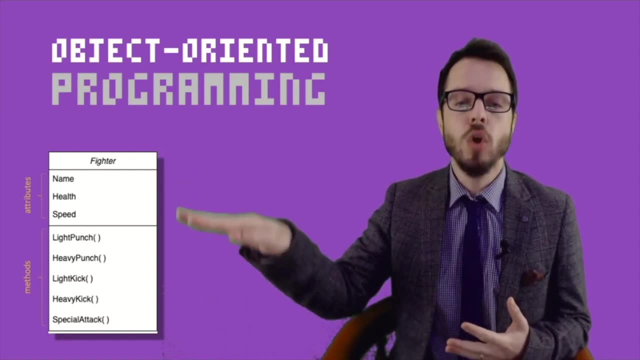 So just keep these things in mind, right? But this thing right here is not not an object yet, right? So this is just a description, This is just a blueprint of what every fighter object in our game is going to kind of look like. 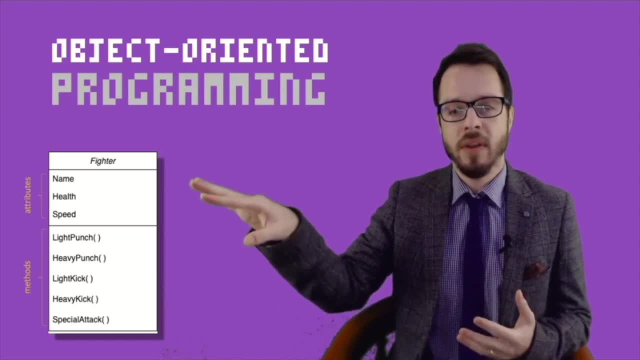 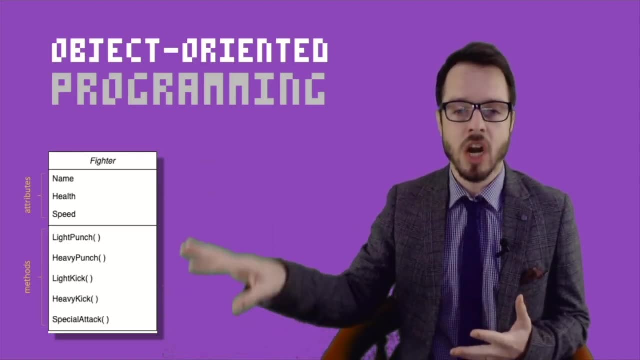 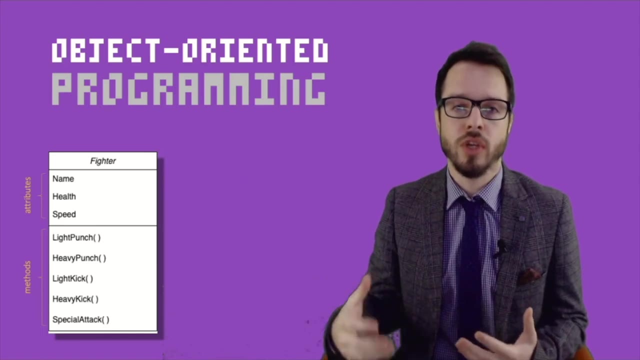 and be able to store and invoke. Whenever we are declaring this blueprint right here, you will see that we're going to call this thing right here a class, right? So classes are these basic descriptions of all the attributes and the methods that our objects of the type fighter are going to be able to store. 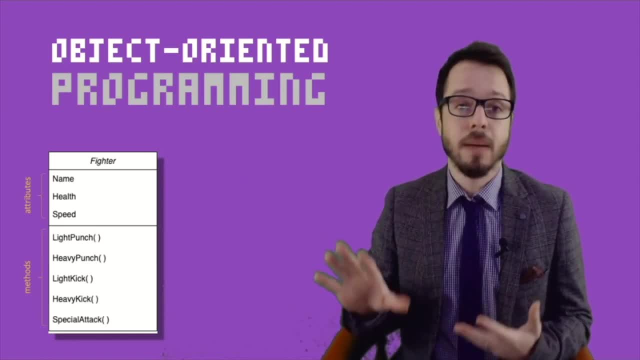 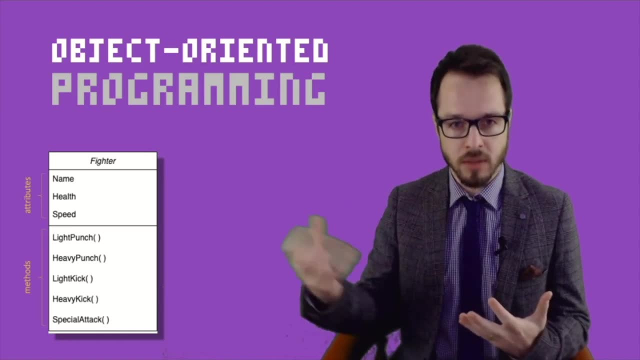 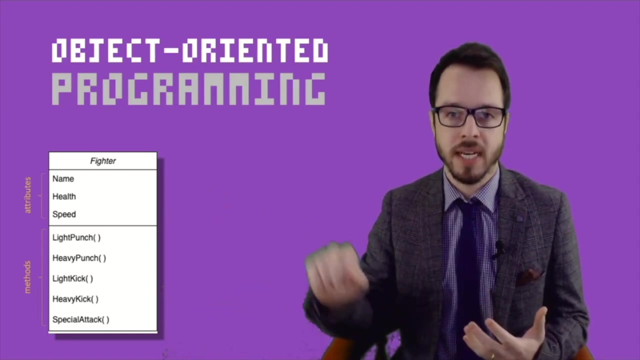 And invoke. Okay, So a class is a blueprint, right? The same way that you can have one blueprint and create several houses based on that blueprint, We are going to be able to use one class to create several different objects of that class. 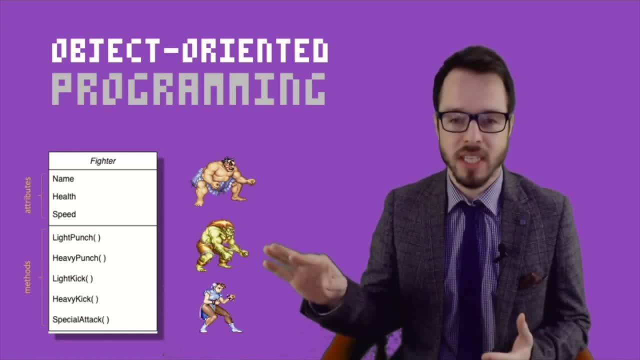 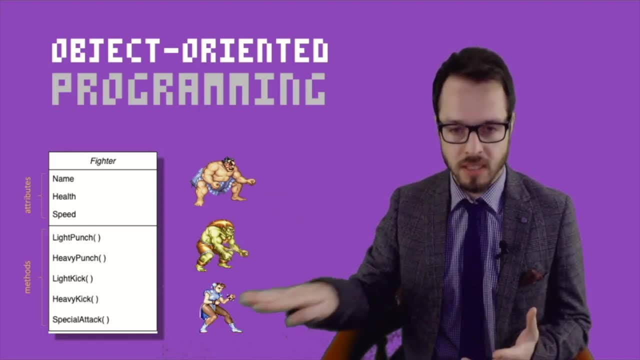 So just to put things into context again, let's just say that I have this fighter, this fighter and this fighter. They are different fighters, right? So this thing is different than this and this different than this one. right here they are special, unique objects of the type fighter. 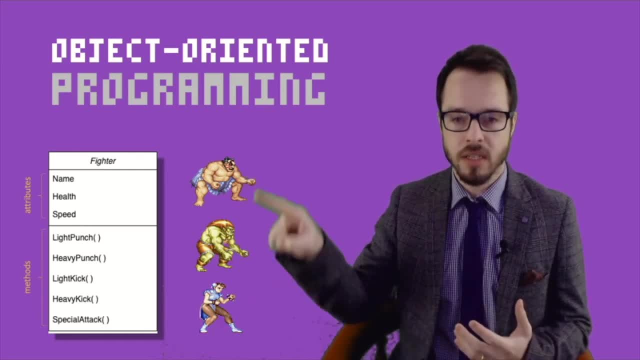 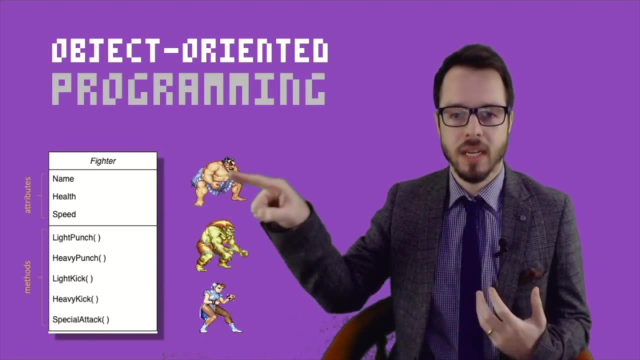 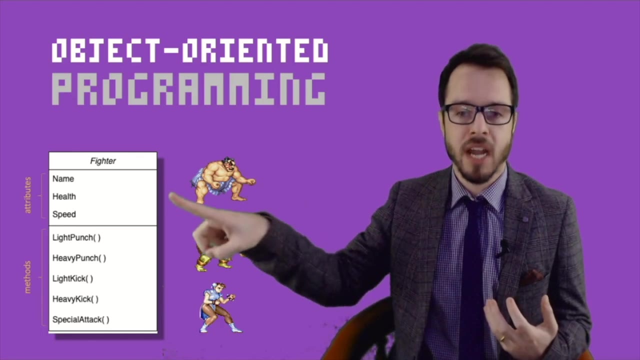 but this thing, this thing and this thing right here, this object, this object and these objects, they will be all of the same class, right? so this thing right here, which is the honda fighter, right, the honda fighter is going to be an object of the fighter class blueprint, right? so this is an object. 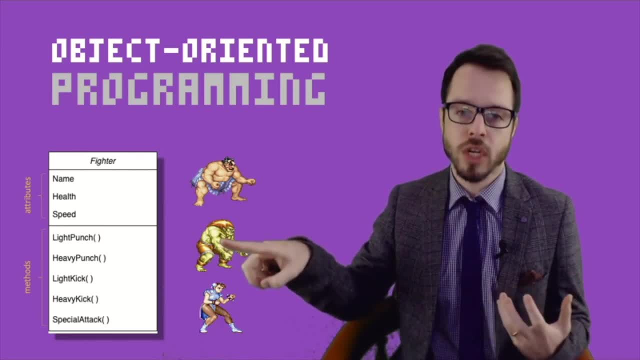 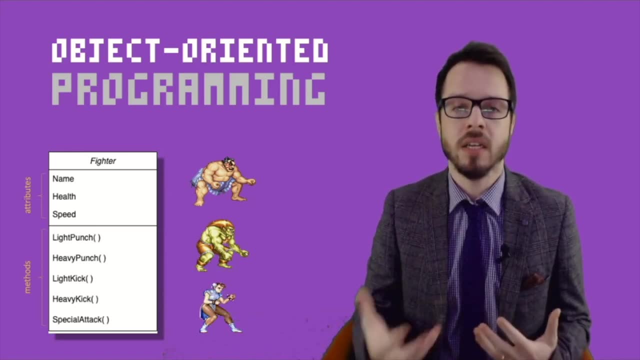 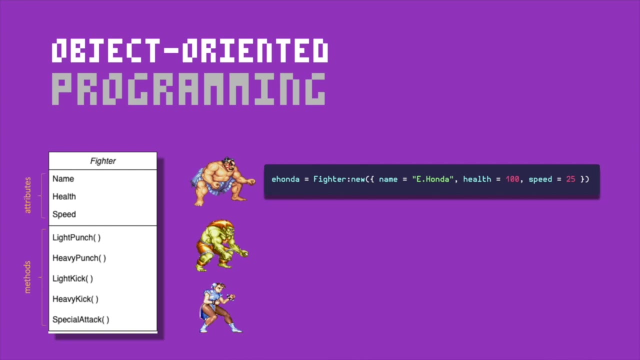 of the class fighter. this thing right here is also an object of the class fighter, and this right here is an object of the class fighter. so whenever i am trying to declare these things as objects of a certain class, of a certain blueprint, you will see that in lua i can simply go and say e honda, right. 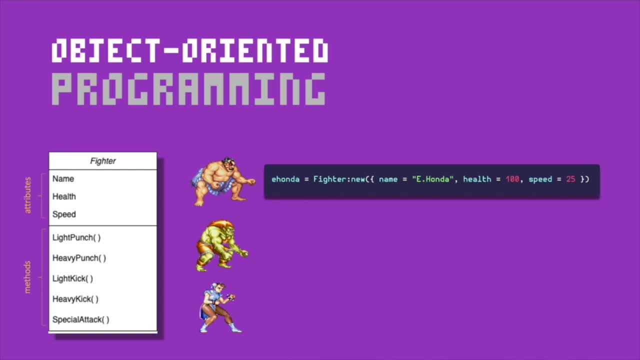 the name of my object i'm creating an object is equal to fighter colon new. so whenever i say fighter colon new, i am calling the constructor method to create a new fighter And I can even pass the parameters of how I want to initialize the attributes of that object. So eHonda is equals to fighter colon new And you. 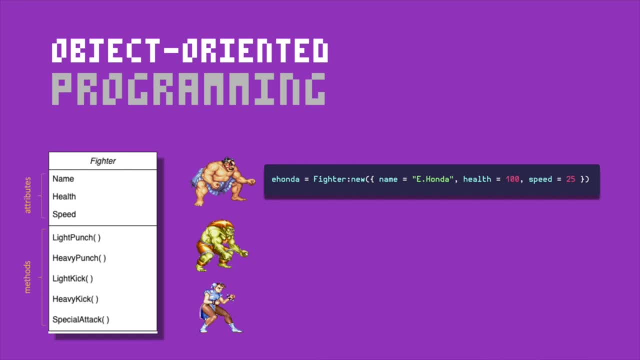 will see that this colon notation is something that is very unique to the way that Lua works with objects. So fighter: colon new, And then I can open parentheses and start passing a little table with the attribute values. right? So key value, key value for the attributes and values. 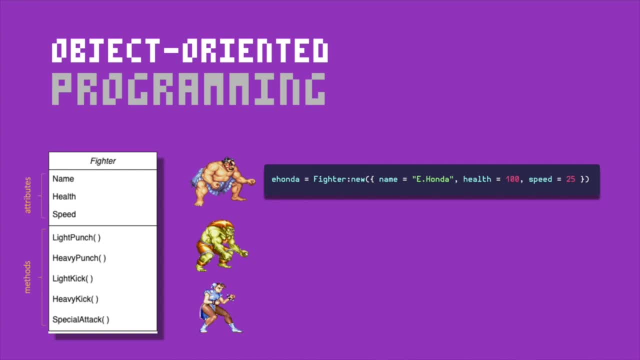 So I can initialize my object with the name eHonda. I can say that the health starts with 100 and the Honda speed is 25, right, Let's just say that it's very slow. So this is us creating an object of the class fighter and initializing the attributes with certain values, The same way that 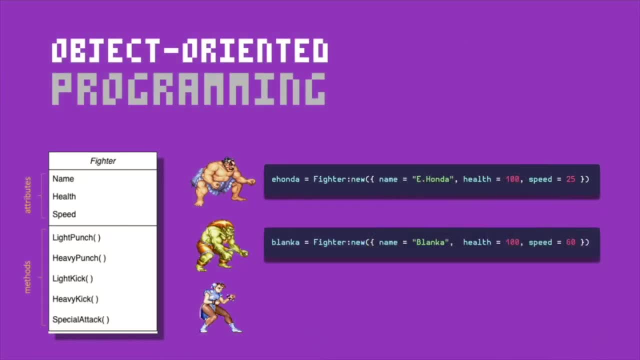 I created an object of the class fighter called Honda. I can have a new object, also of the class fighter, but then this object is going to have different attribute values. I can initialize it with the name Blanka, The health is 100 as well, And then the speed is 60.. 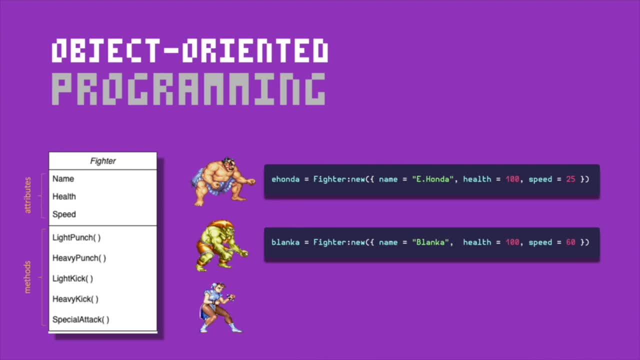 So let's just say that's a little bit faster than the Honda object. And you know, right, Same thing I can have now Chun-Li, this Chun-Li object that is also of the class fighter, And I can call fighter colon, new passing, the name Chun-Li, the health 100 and the speed 85.. 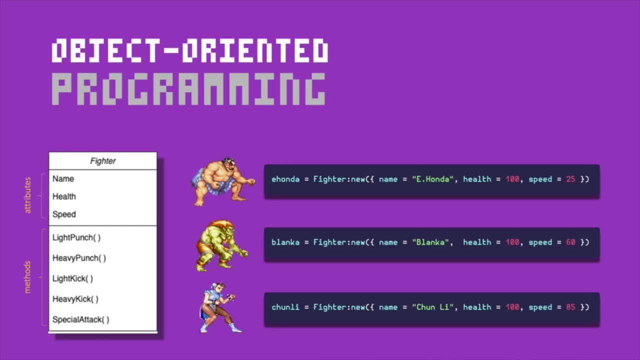 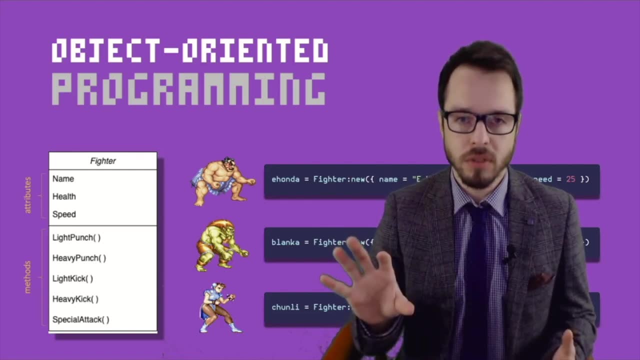 Let's say that Chun-Li is a lot faster than all the other characters, So I know that this is very high level, right, But I just wanted to understand that we're going to have all these concepts of attributes, meaning the data that our object can store, And we're going to see how we can declare. 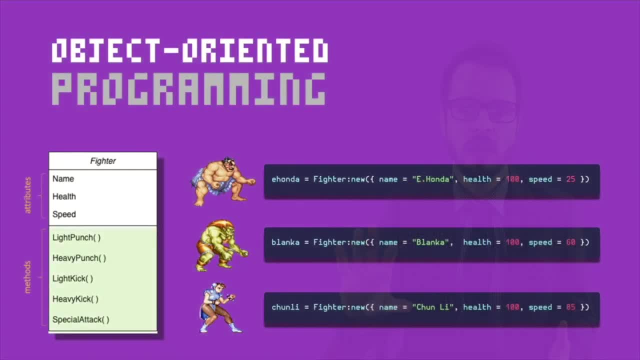 now the methods right. So what are the functions? What are these little calls that our object can invoke? Light punch, heavy punch, light kick, heavy kick. So these are the methods that we're going to be able to invoke. Perfect. 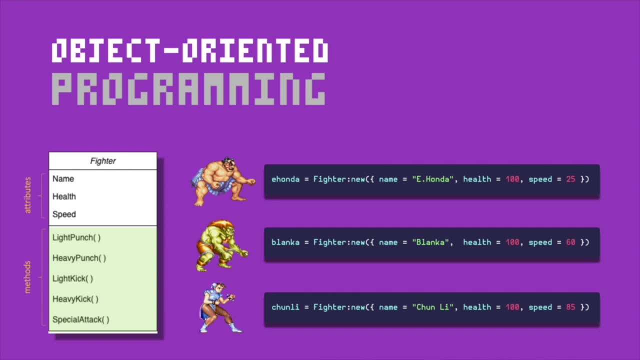 So I'm going to show here on the screen an example of how we can declare a class and how do we define. what are the attributes, what are the methods that this class fighter, for example, is going to have. So I'm going to have to declare a class fighter that has the attributes name, health and speed. 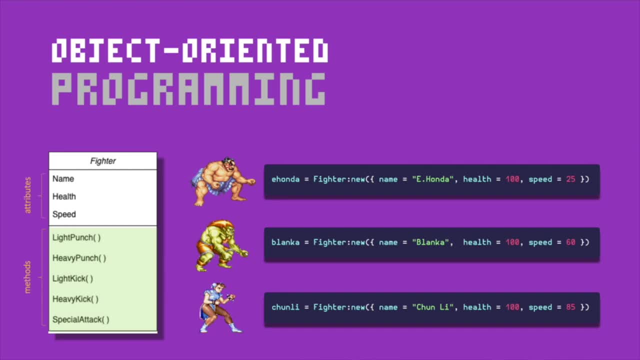 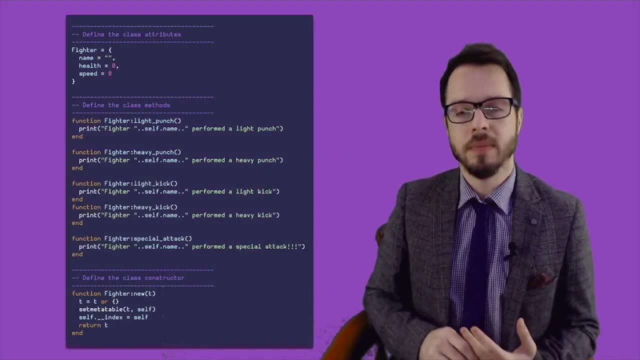 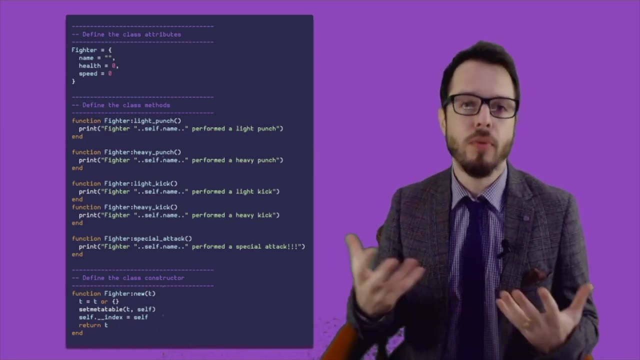 and has the methods: light punch, heavy punch, light kick, heavy kick, and etc. So let's look at the Lua code that will make this possible, Right? So right here on this slide, I have a full code. that is the declaration of my class, right? The declaration of my object: blueprint. 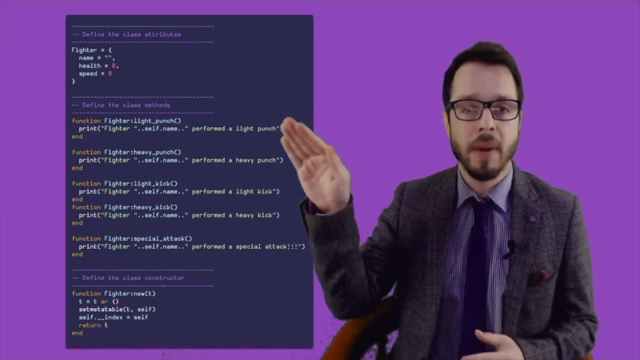 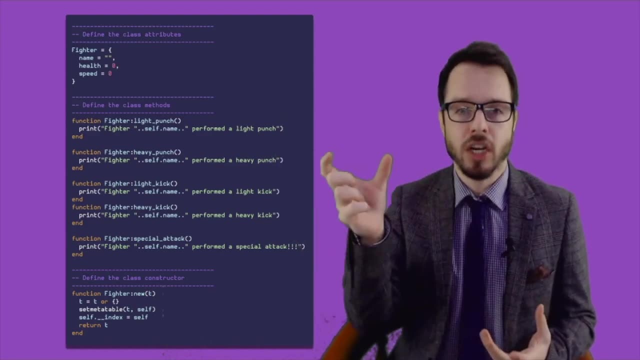 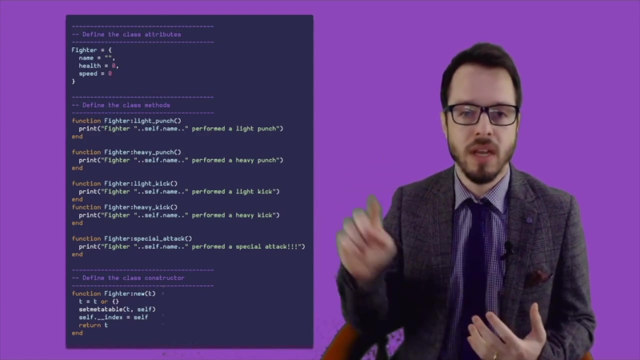 So the way that we start these things is: first I can start by defining the little table with the attributes, right, So I can say: define the class attributes, and then I say fighter And you will see that traditionally I name my classes with this uppercase right. So fighter is going to be. 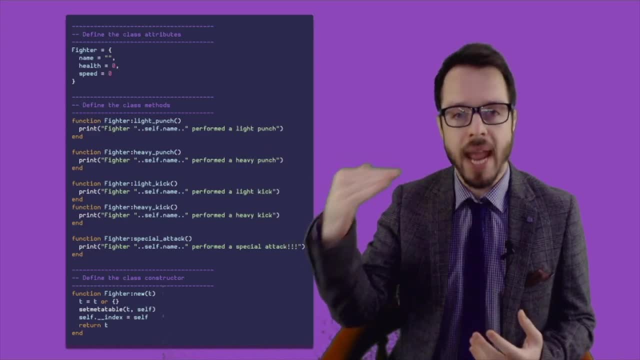 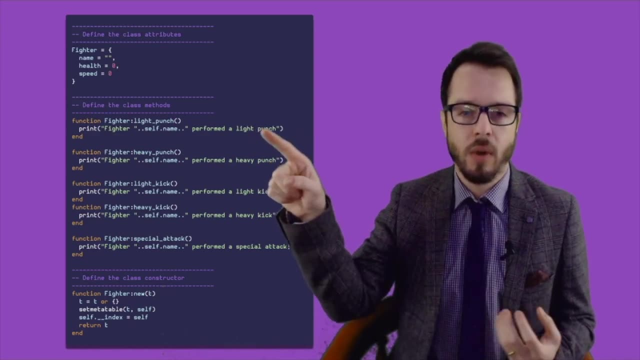 a class And this class I can initialize with the attributes that the class is going to have. So I'm going to initialize with the attributes that those objects are going to be able to hold right, So I can initialize with name. So you'll see how I am initializing name with empty. 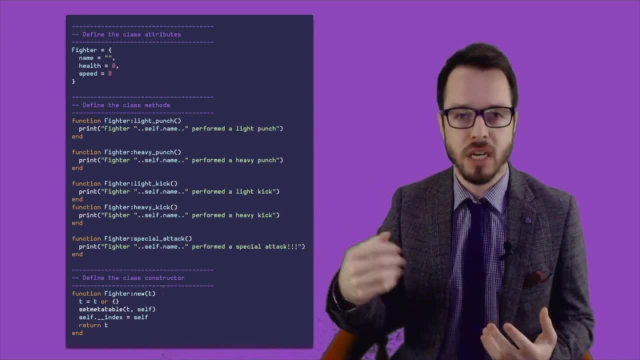 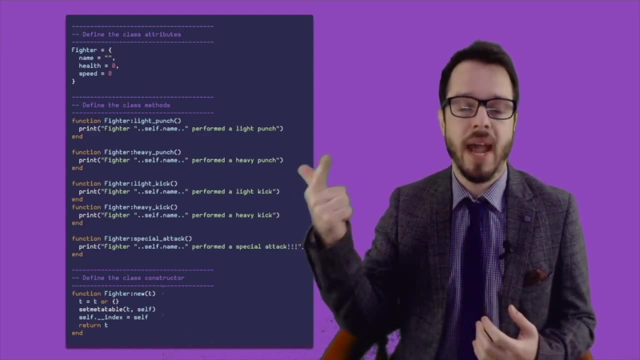 That is just me kind of cleaning the attributes, right, So I'm just kind of initializing them with some empty values. So fighter class is going to have name, is going to have health, which is going to be a number, as you can see by me initializing there with zero, and also speed. 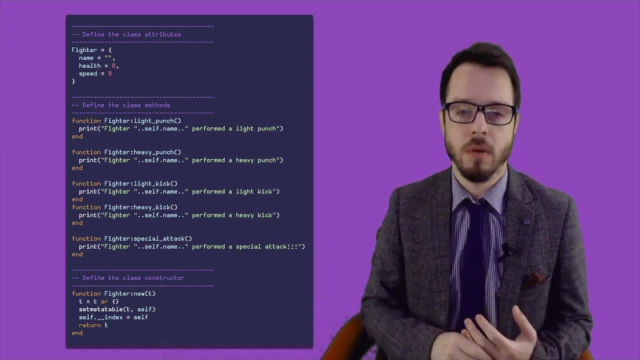 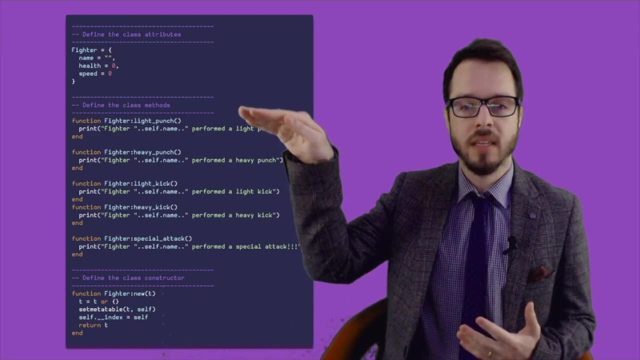 right. So speed is also going to be a number, because I just initialized that with zero. That is me initializing the attributes of my class And now I can come here and I can start adding what are going to be my class methods, right? So what are going to be the little? 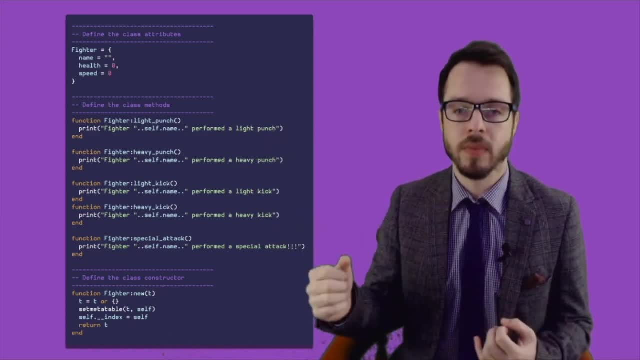 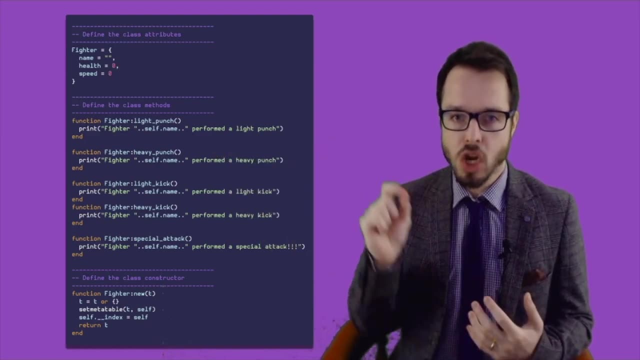 functions that I can invoke as my object: methods. So, as you can see, here I can say: function: fighter colon, light punch. Remember when I said that the colon was very unique of the way that Lua worked with these ideas of methods. So class: colon, the method name: fighter colon, light punch. 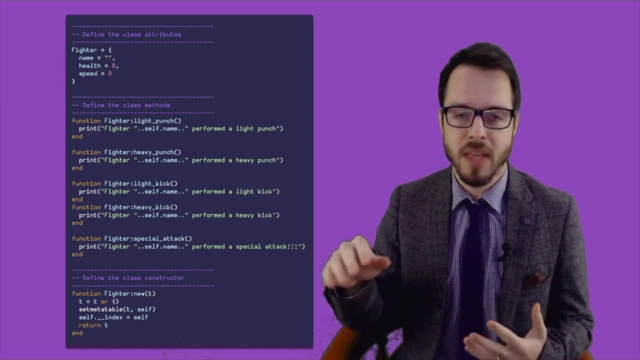 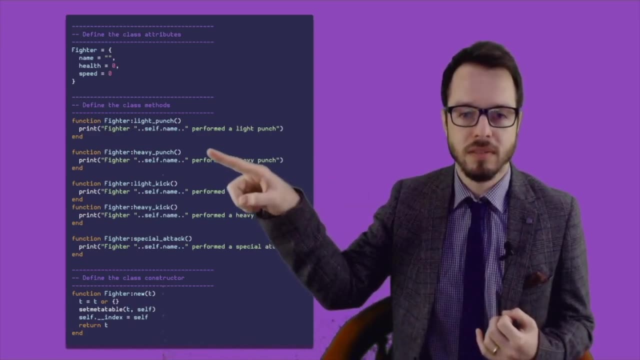 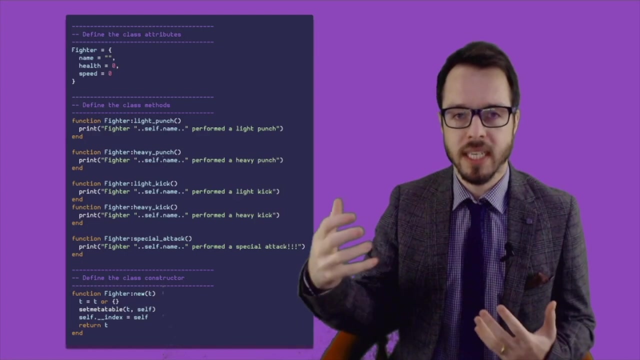 For now, all I'm doing is I'm not actually implementing anything, I'm just printing something on the screen whenever we invoke that method, right? So print fighter selfname performs a light punch Selfname. we are going to understand this a little bit better later, but 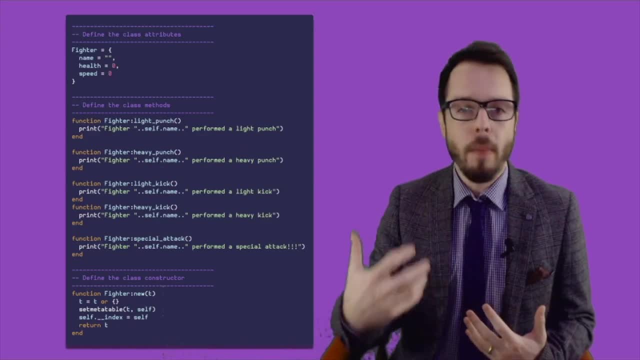 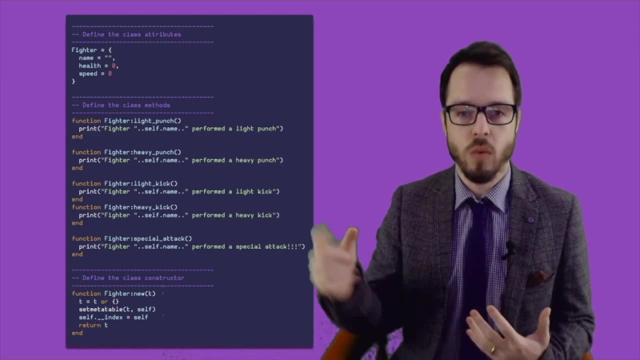 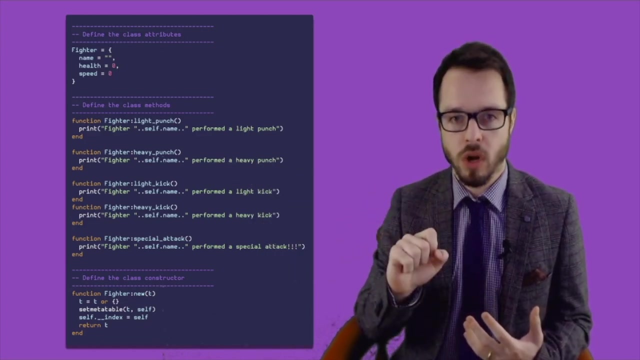 whenever we invoke a method, the object is the one responsible for calling the method. So whenever a method, we have access to the actual object that was the one that called that method by using the little self keyword. so if I say self dot name, I'm going to 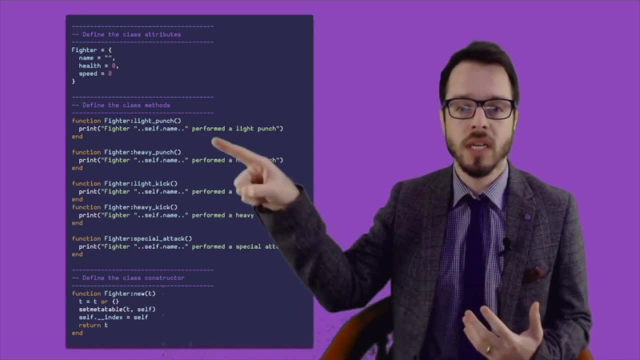 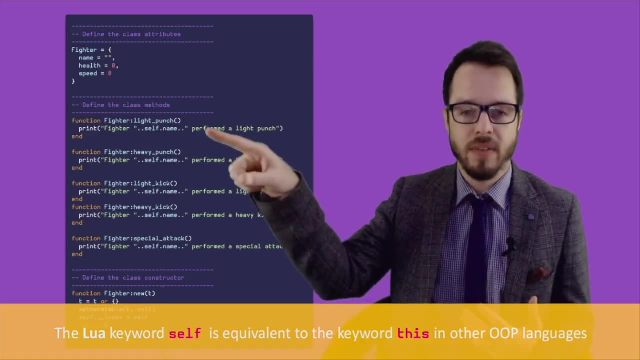 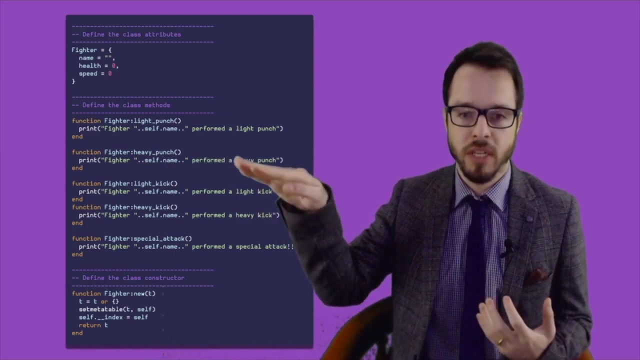 get the name attribute of the object that just called this function right here. don't worry, we're gonna see this very soon of how these things work right. so I declare a method and these ones right here: exactly the same thing. I'm declaring a new method: fighter colon heavy punch, which is just print. 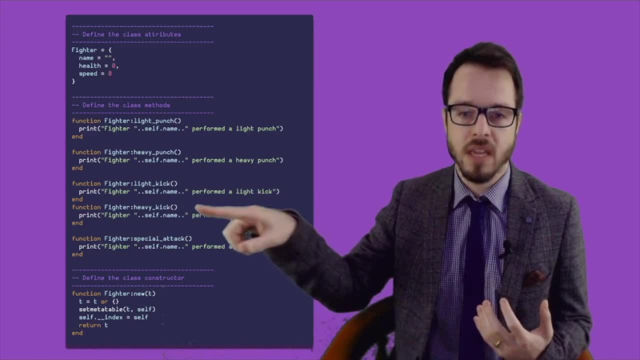 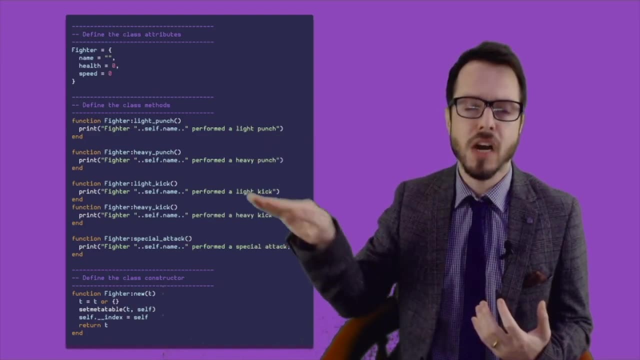 something: the light kick that just print something, the heavy kick that just print something, and also the special attack that just print something. so I have all these little functions that are going to be actually methods of my object- and this is how I declared- and the attributes, and this is how I. 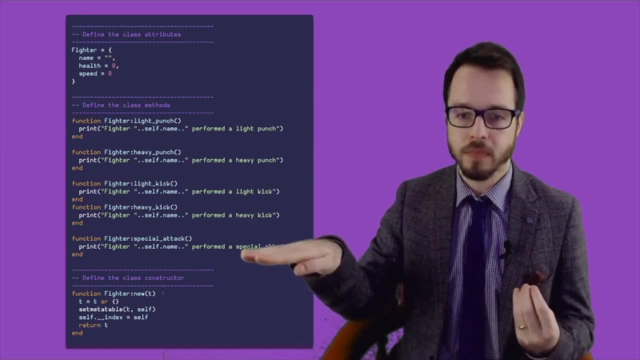 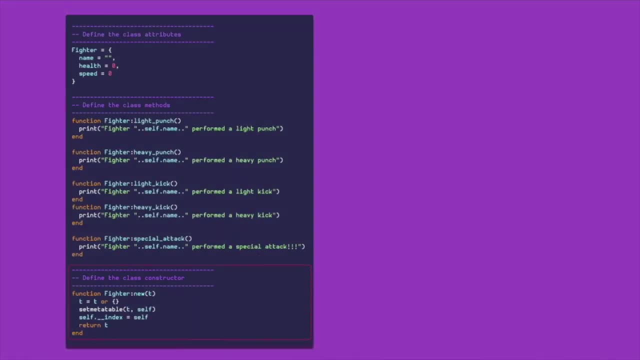 declared the methods of my class, right, of my blueprint, and right here, this is what Lua uses. right, so Lua uses this concept of a meta table to kind of bind these things together. right, so I have what we call a class constructor method. right, so I can say: 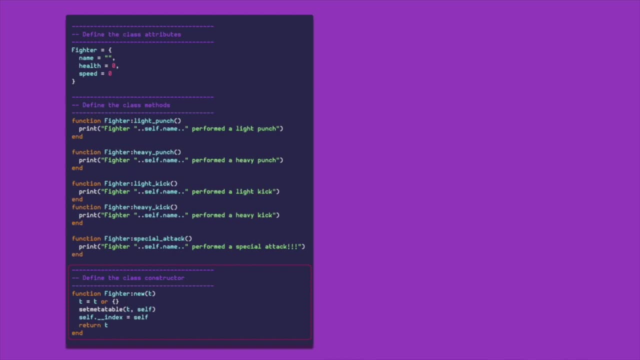 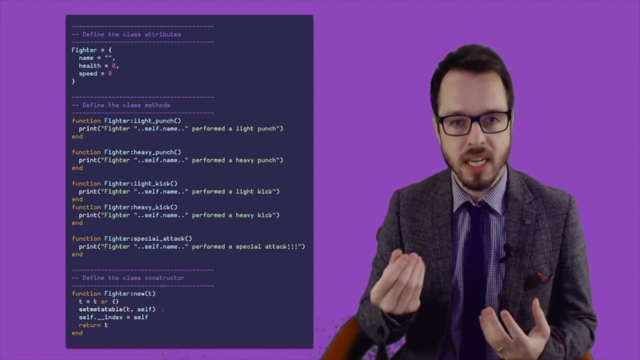 fighter colon new, and then I pass a little T as parameter. I have to pass a little table as parameter. I have a very special syntax there that says T equals T or open, close, curly braces. this is a very special Lua syntax. it's like a syntax sugar thing that says T will receive the value of T if T is not nil. 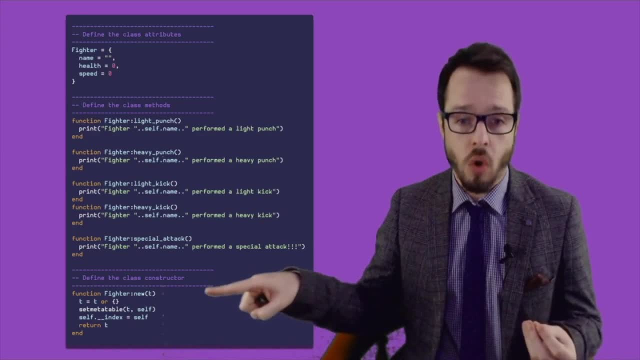 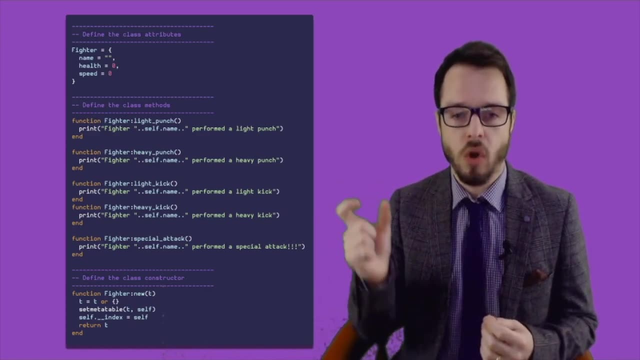 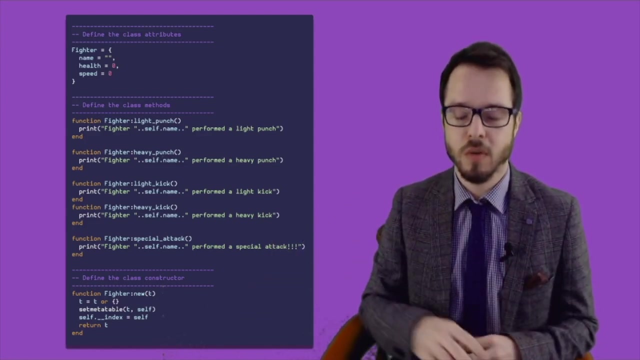 if T is not nil, and if it is nil, I will go to the or and assign empty curly braces. so it's basically saying T is equal to T or curly braces. if T is nil, then I assign the empty curly braces table. alright, so this is something that you see. 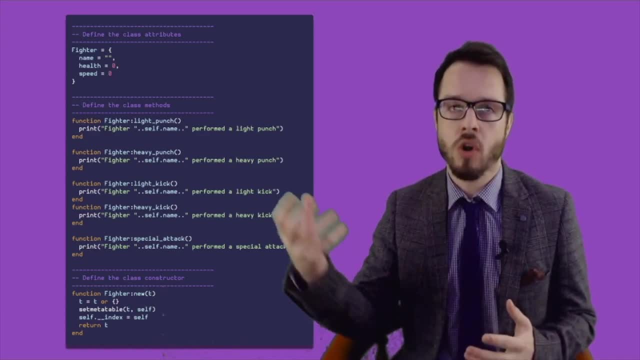 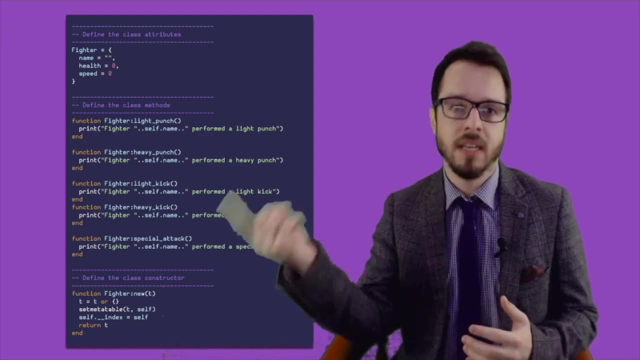 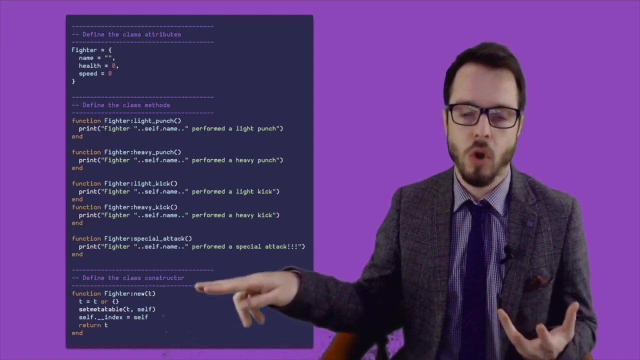 sometimes, as used in Lua, right, so T is equal to something or curly braces. so if, by any chance, the thing that we are trying to assign, it is empty, if it is nil, then I assign the second option. right, I curly braces. Okay, so t. the parameter is going to be not new, hopefully, right? So then I assign. 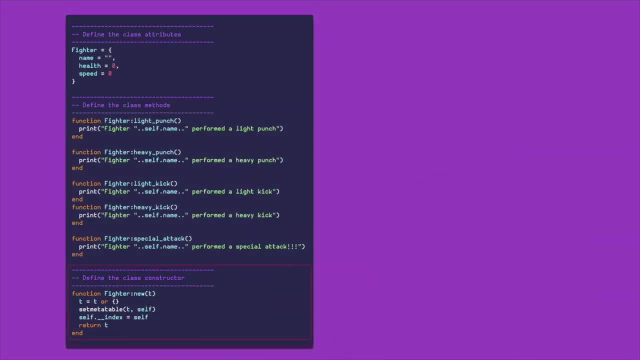 t to the table, I create the bind between my meta table and my table. So I'm going to bind the set meta table t with the self object and then I say self underscore. underscore index equals to self. This thing right here is what actually creates these ideas of binding methods and binding the 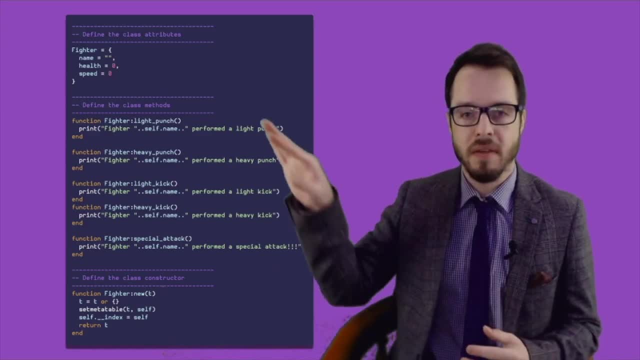 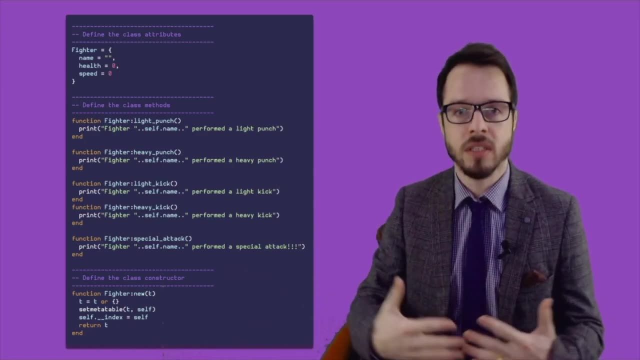 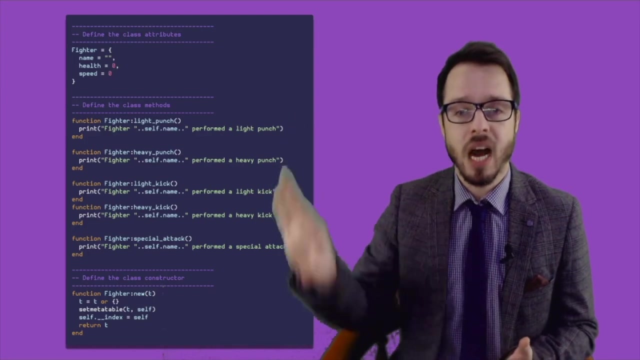 attributes in this object idea of Lua, right? So I have the attributes, I have the methods, and then- here is where I actually make things happen. I actually bind the methods and the functions and the attributes in this little new object that I create. okay, So this is how we. 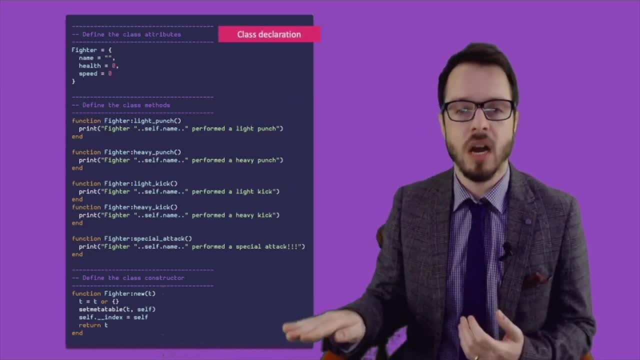 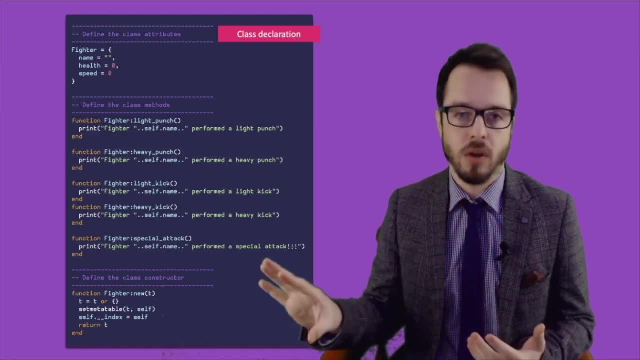 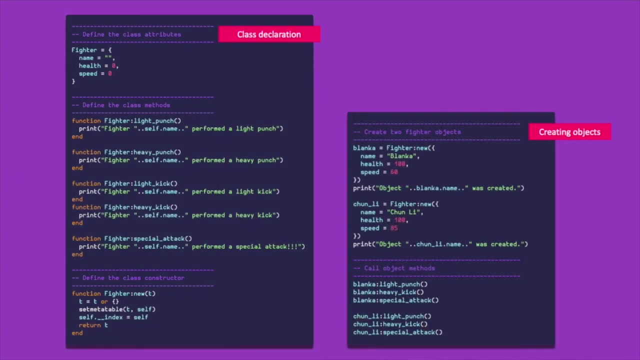 create a little class declaration, right. So all these things right. here is how we declare attributes, methods and then the constructor, right. But this is not enough right? This is just the blueprint of our object. We need to be able to now go and create the objects themselves. A class is just a blueprint. 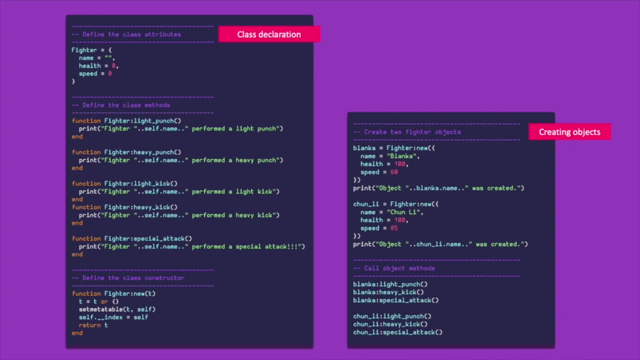 I need to use this class to go ahead and actually create objects of the type fighter. So here on the right, I have a couple of examples of me creating objects of the type fighter, or you will see programmers call this instantiation. right, I'm going to instantiate an object of the type fighter. 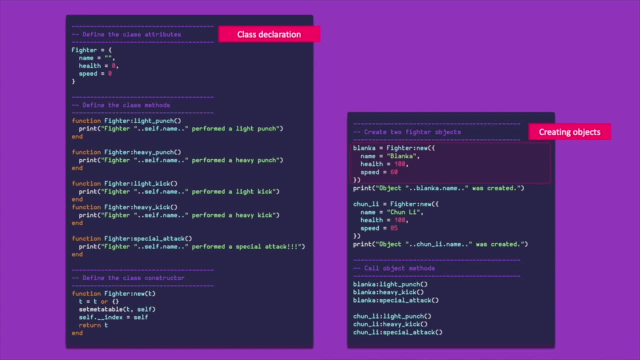 So in the first part of the code I am creating objects. So you can see that I'm creating blank which is equal to fighter colon new, and then I pass as a parameter the attributes that I want to initialize the object. blank with So name equals blank: health 100, speed 60.. As soon as I'm done. 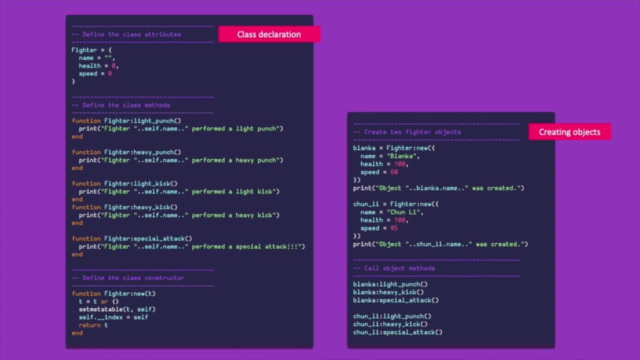 calling the fighter colon new. I print object: blank dot name was created So I can have access to the little attribute by saying blank dot name. okay, So I'm not hiding the attributes inside. This is an example of a class that has the attributes public. I can say blank dot. 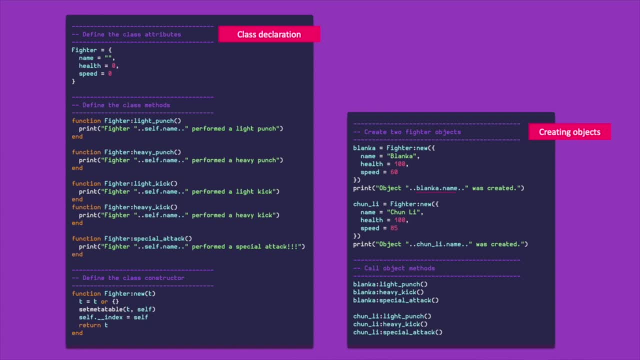 name. This is how I access the attribute inside my blank object. So as soon as I'm done creating the blank object, I go ahead and I create a new object of the type fighter, So Chun-Li equals fighter, colon, new with the attributes of Chun-Li, So name Chun-Li, health 100, speed 85.. And as soon 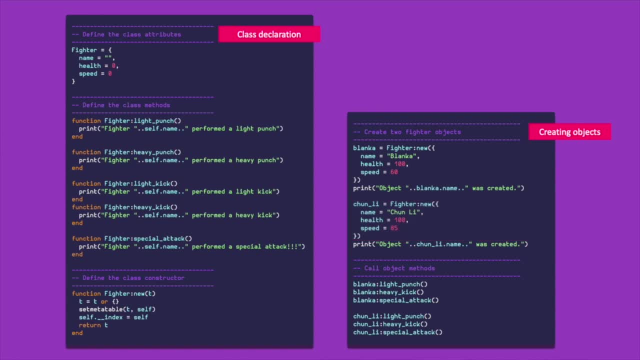 as I'm done. object Chun-Li dot name was created, So these two calls are me calling the constructor and creating two objects of the class And, as you can see here on the bottom, I can also start calling the object methods, right. 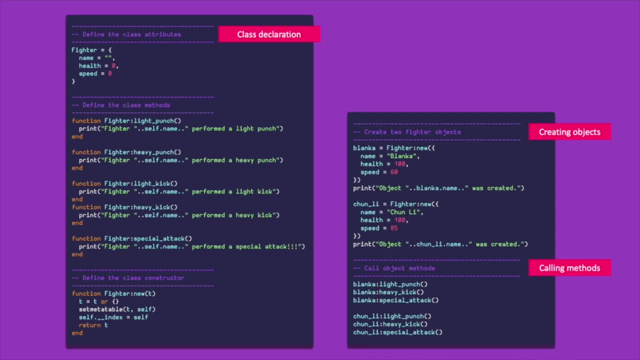 So look how my object is the one responsible for calling its own methods. Blanca is calling the light punch, Blanca is calling its heavy kick, Blanca is invoking its special attack. So this is not a normal function call. Do you see? that is the object colon, the method name. 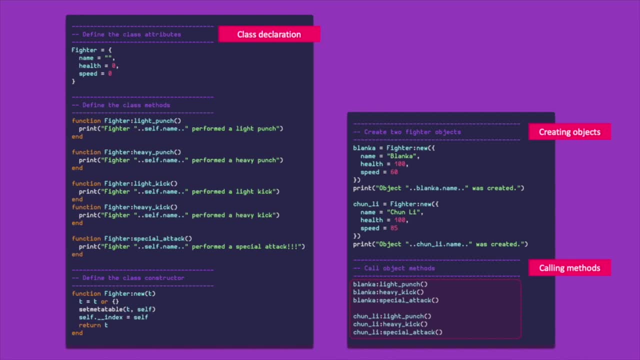 I am using the object to invoke its methods, And I can perform the same thing with Chun-Li. So I can ask Chun-Li to perform a light punch, I can ask Chun-Li to perform a heavy kick, And I can ask the object, Chun-Li, to perform. 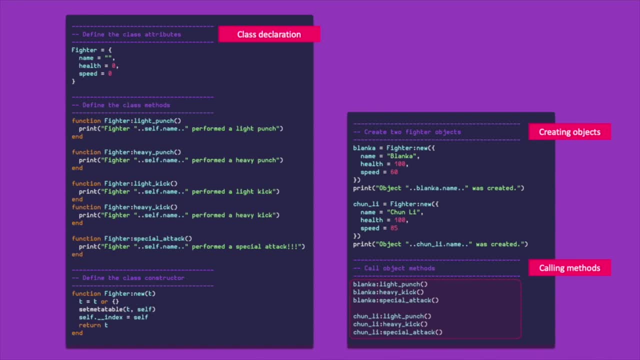 its special attack. This is extremely important. The objects are responsible for calling their own methods, And this is one of the powers of object-oriented programming. As we start coding with these things, you will see that this brings a lot of power to us. So just a quick review again. 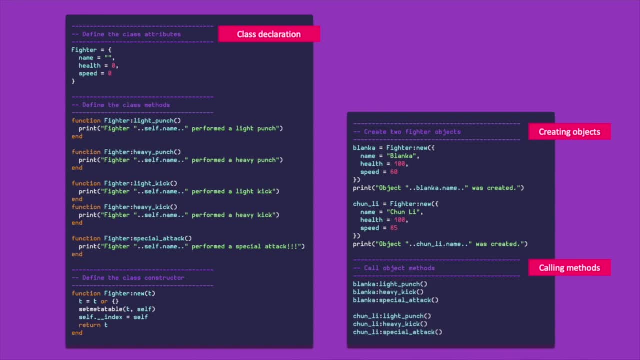 On the left we have our class definition. right We define, we declare our class, The blueprint that is going to be used to create fighter objects, And on the right, I am actually creating the objects. by calling the class colon new, passing the attributes, I create two objects And as soon 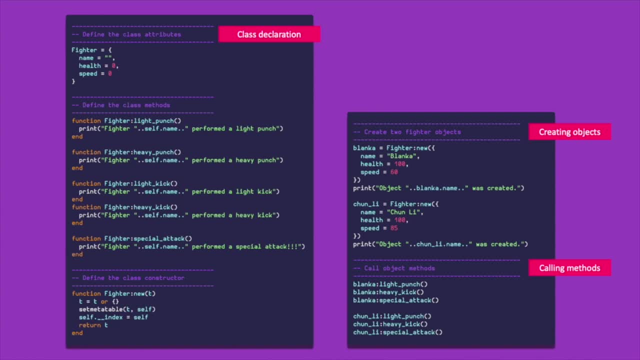 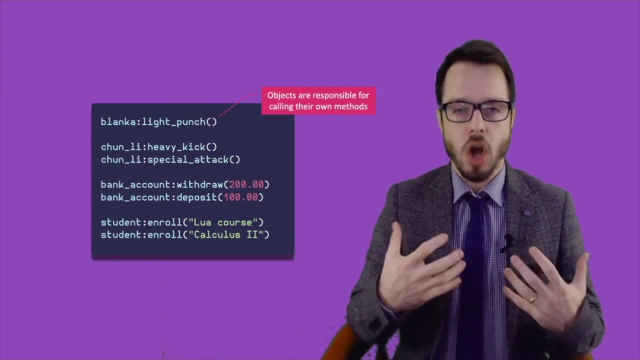 as I'm done, creating the objects, then I'm free to go and start invoking and calling their methods, which are basically those functions that we declared before, And still talking about this idea of the object being responsible for calling their own methods, I just put a couple of examples. 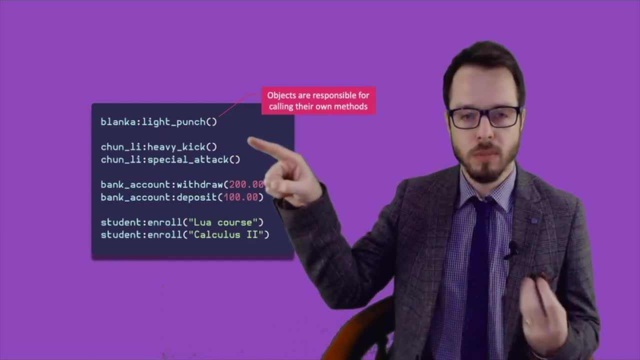 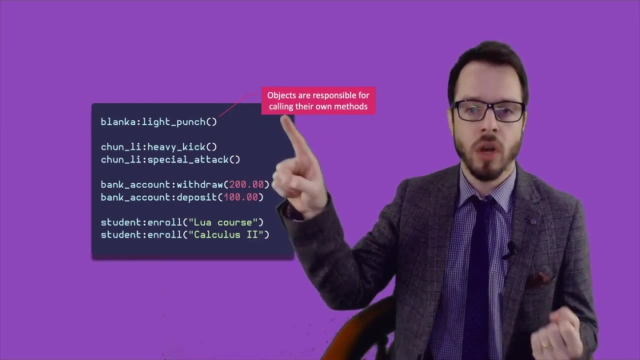 here. So remember how Blanka was the one responsible. The object, Blanka was the one responsible for invoking and calling the light-punch method. So the object is responsible for calling its own methods. Chun-Li was the one calling the heavy kick. Chun-Li was the one. 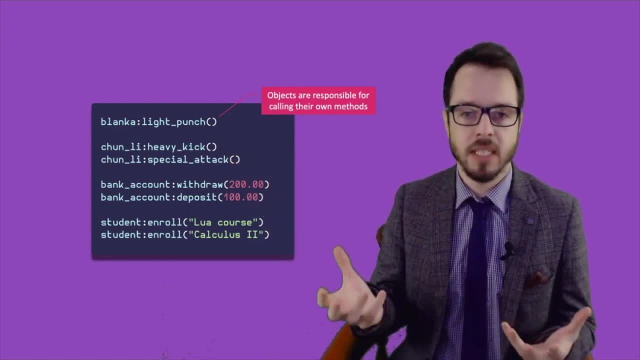 calling the special attack. Let's just say that I have in my system a bank account object, So in a bank account. do you agree with me? Do you agree that we're calling it in ajs? Do you agree that we would be primarily charging in живão? But actually we don't know why this might be said like this. 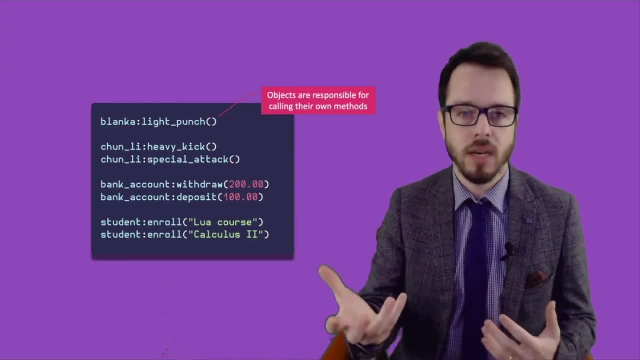 Formretch is a kind of property. if you have milk farming and softwares, everything is industry or demilitarization. of persuasion, However, like this is point in time right. So our goal is not from a basis that it will be beneficial for us to be able to ask to withdraw a certain amount from a bank. 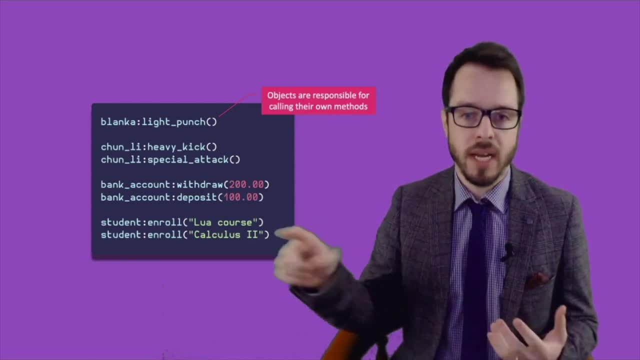 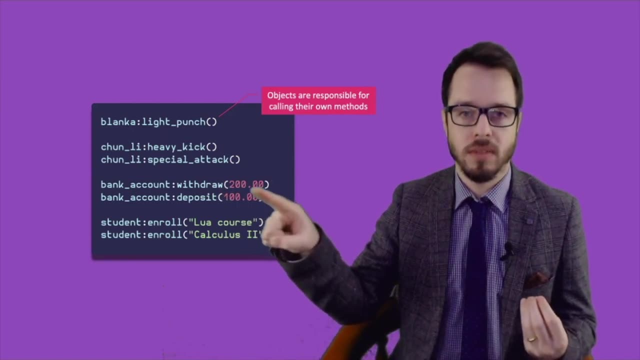 account or even deposit an amount. So the way that I would do that is, the bank account object- is the one invoking the withdraw method, And I can pass parameters in the methods as well, if I want. So what is the amount that you want to withdraw from the bank account? Let's say that I want to. 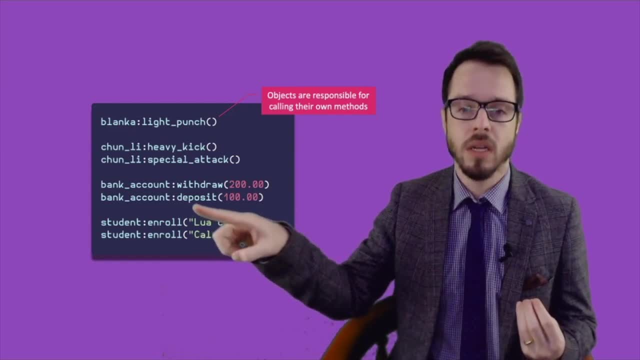 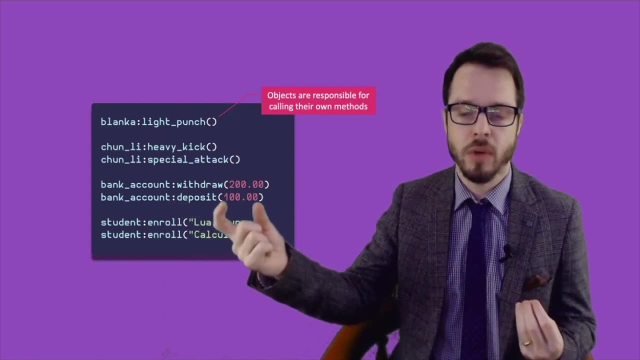 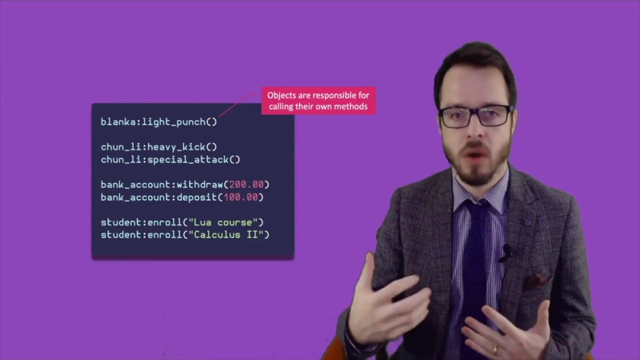 withdraw 200. Or bank account colon deposit. So I am invoking the method deposit from the bank account object And I can say how much I want to deposit in that bank account. So the object is the one that invokes that calls the method on its own data. Let's say that I have a student object in my 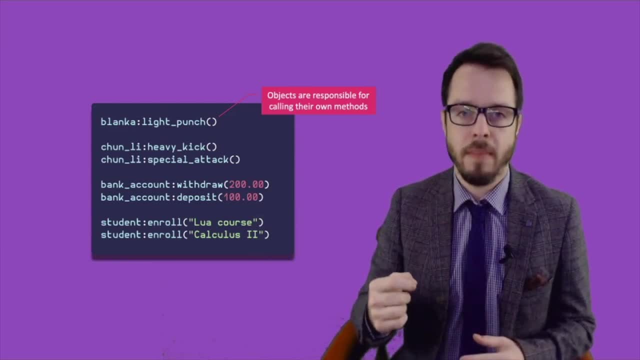 system I can say student, and students usually will have a method called enroll And I can even pass a little String value of what is the name of the course that I want to enroll. So I can say student enroll in the Lua course And then I can have student enroll in the calculus 2 in the university or 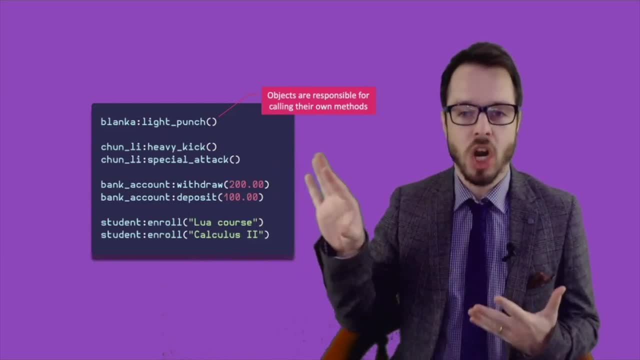 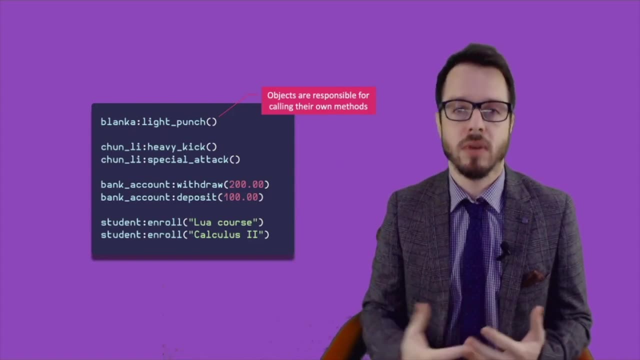 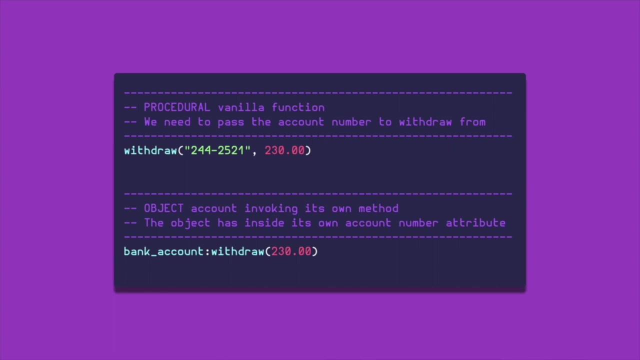 something like that. So again, objects are the ones responsible for invoking and calling their own methods. So that is how I have to see things right now. It is not a vanilla function that I can just say: withdraw a certain amount And then I have to, inside the function, decide the. 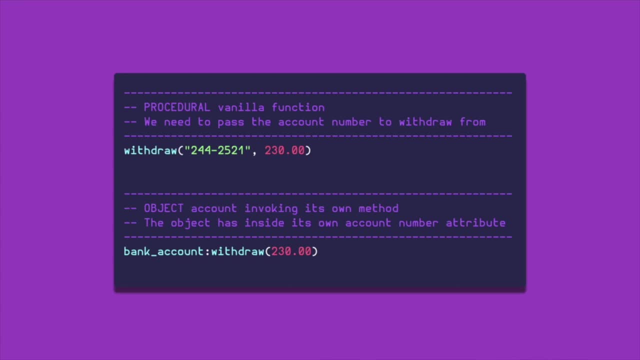 value of the method. So that is how I have to see things right now. variable that I have to withdraw from In the object-oriented world, my bank account. object is the one invoking the methods and then, if I want, I can pass parameters or not, right This?